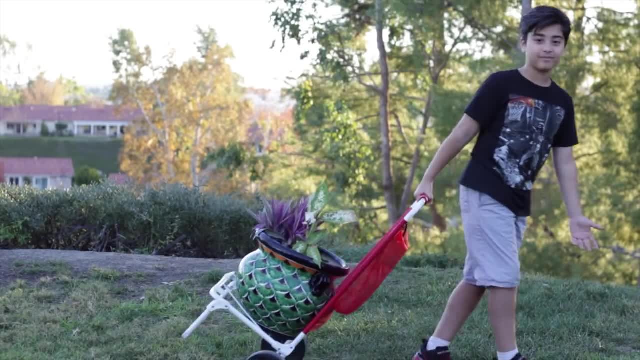 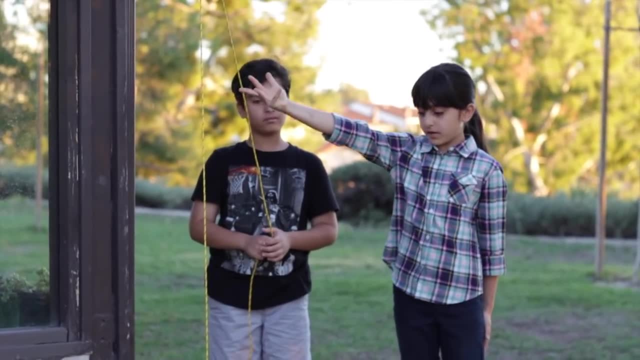 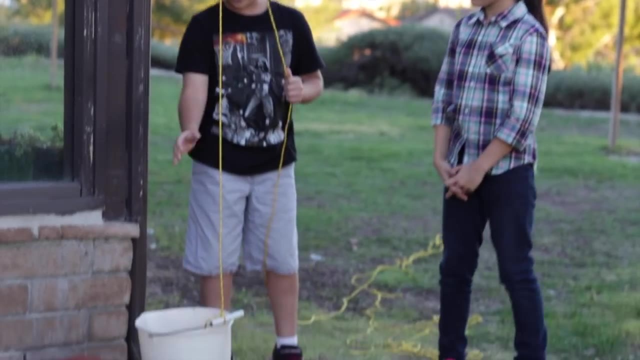 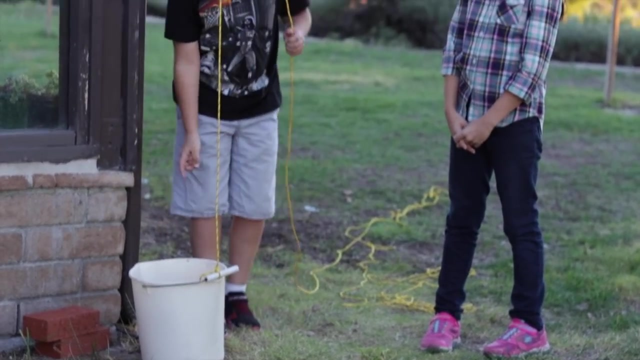 I can easily do this with just one hand. This is called the pulley system. This is used everywhere, but it is used especially in construction. Now, over here, in the pulley system we have, we have three parts. One is called the load, which is the bucket over here and in the 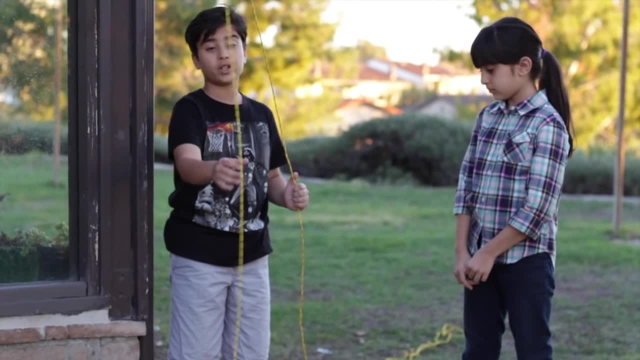 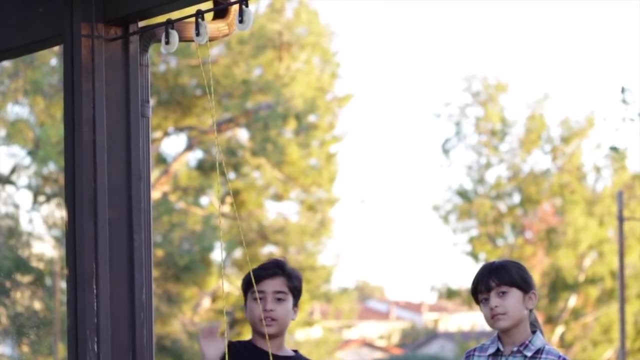 bucket there are two really, really heavy bricks. This part over here is the fulcrum, which is the center of the pulley. We have two other fulcrums over here which count as two other pulleys. Now and then, of course, the rope is. 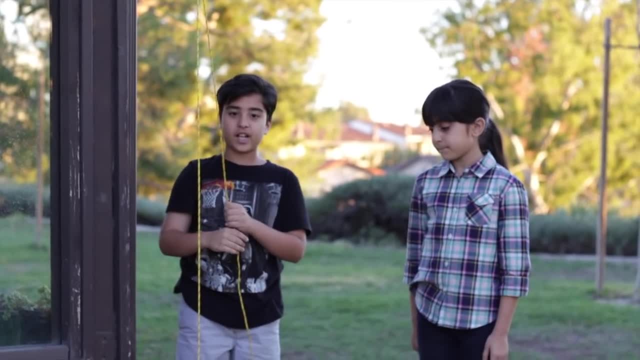 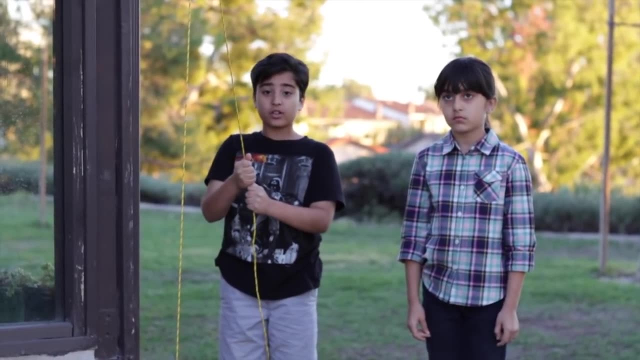 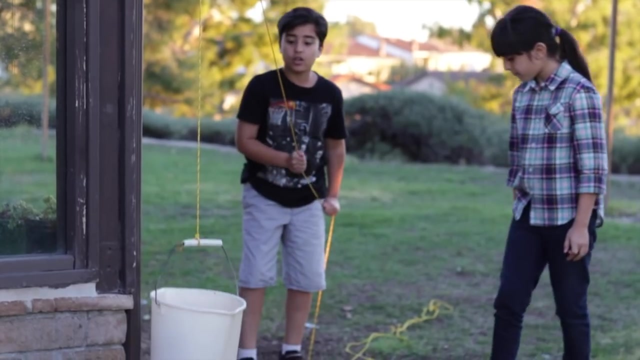 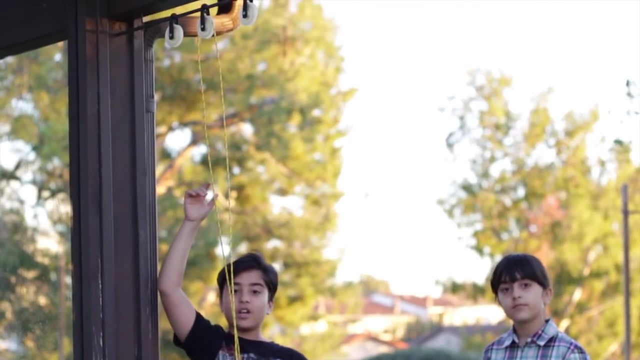 the lever. Now the whole point of mechanical advantage is to create, is to pull the load up. So there are two ways that we could do mechanical advantage. One way is that we could do a longer distance, creating more work with less force. Another way we could do is we could just connect it to more fulcrums so that we could get more rope with less force. 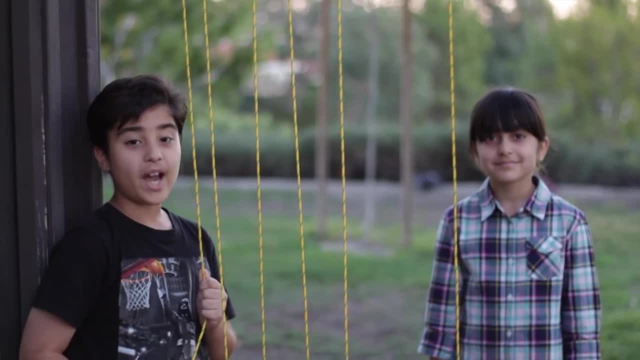 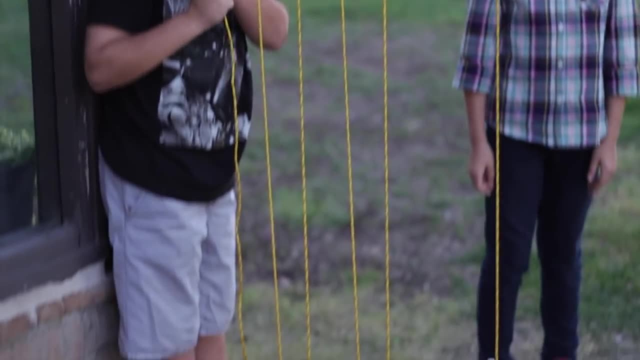 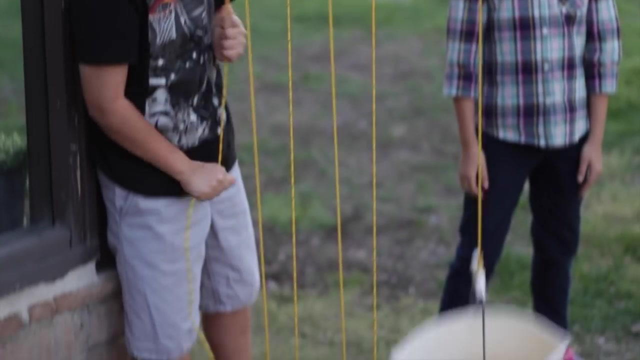 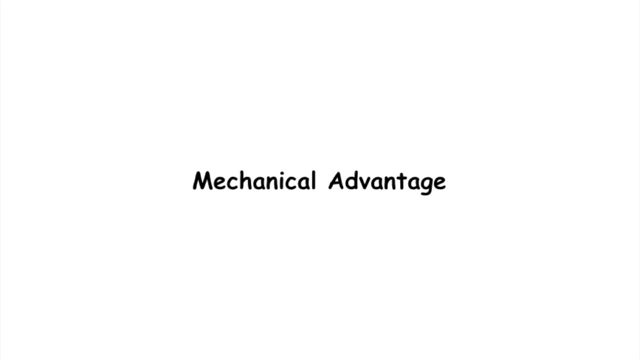 and the same amount of work with just standing in one place. Now we have a full pulley system with six fulcrums, and now check how much easier it is. Before we talk about how the pulley works, we need to talk about a very important formula. 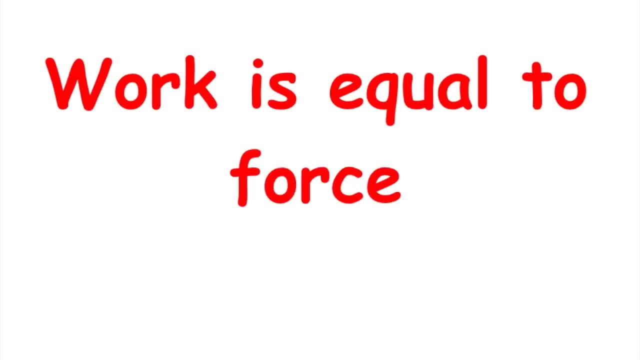 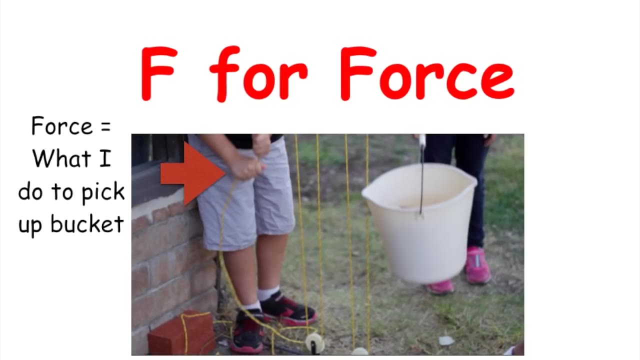 The formula is: work is equal to force times distance, or W is equal to F times D. for short, The first formula is work. The first formula is work. The first part of the formula F stands for force. The force is what I do to pick up the bucket. 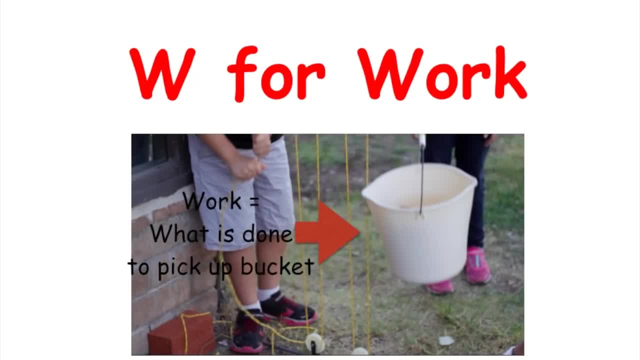 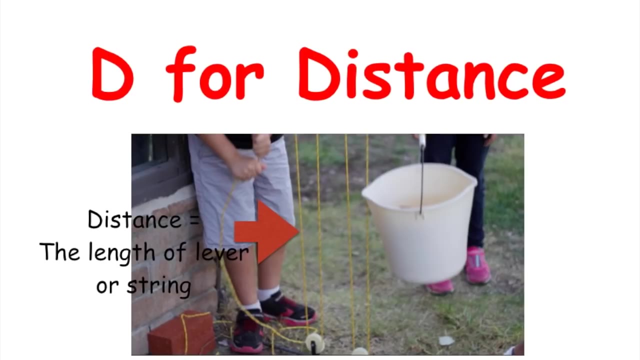 The next part of the formula W is for work. Work is the total stuff that is done to pick up the load, which in this case is the bucket. And finally, D is for distance. The distance, in this case, is the length of the lever, and the lever, in this case, is the string.